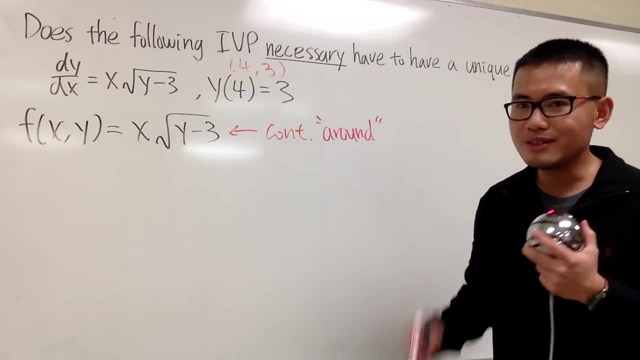 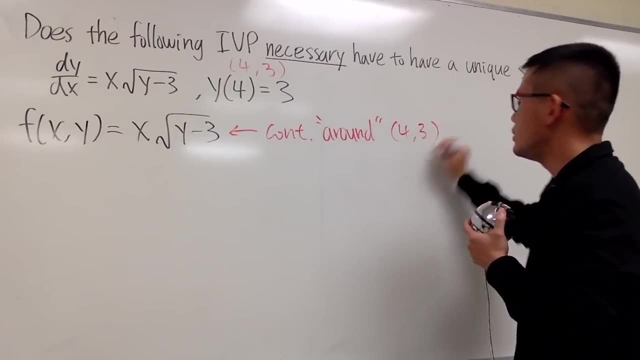 because technically you have to say it's a rectangular region, but let me just use the word around: It is continuous around that initial point 4, 3.. So it satisfies my first check. And now my second check is: 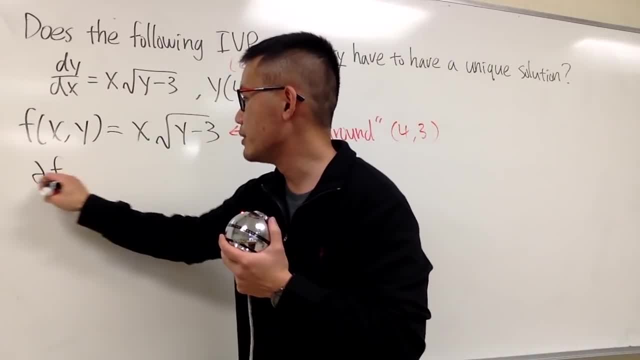 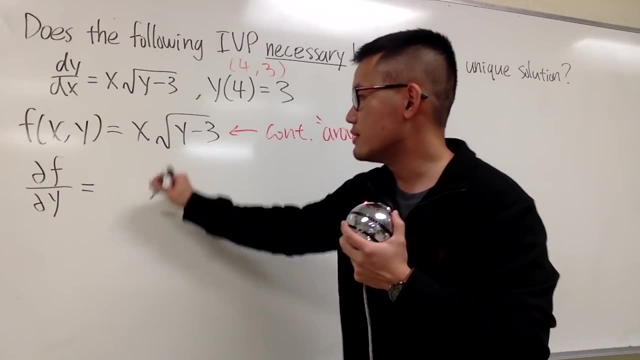 I will do the partial of f with respect to y. So let me put this down, Partial of f with respect to y, And let's figure out what that is first. x will be considered a constant, so we will have that. 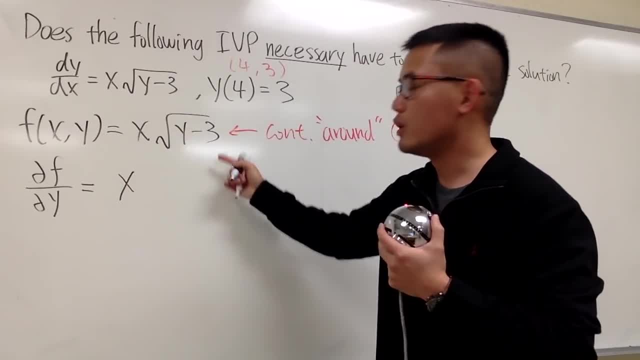 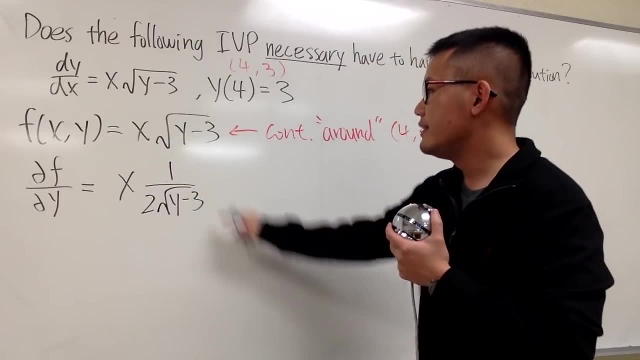 And we have to take the derivative of square root of y minus 3 with respect to y And the answer for that will be just 1 over 2 square root of y minus 3.. And the derivative of y minus 3 is 1 over 2 square root of y minus 3.. 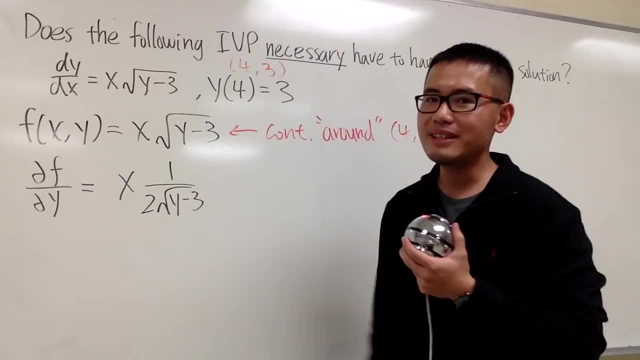 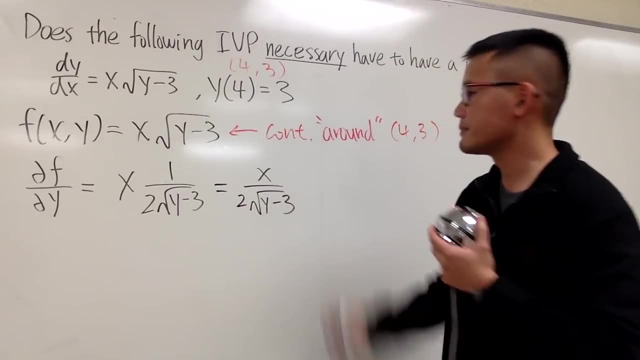 And if we look at the inside with respect to y, it's just 1, so it doesn't really matter, right? So you can just put this down nicely: This is just x over 2 square root of y minus 3.. 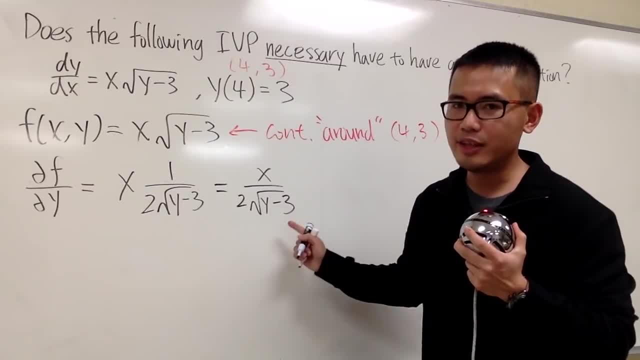 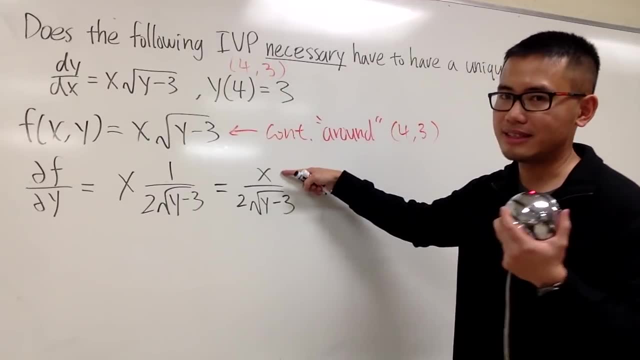 Okay, we will also have to check if this is continuous or not around this point. Well, I can plug in 4 into x. that's nice. However, if I plug in 3 for y, right here I will get what. 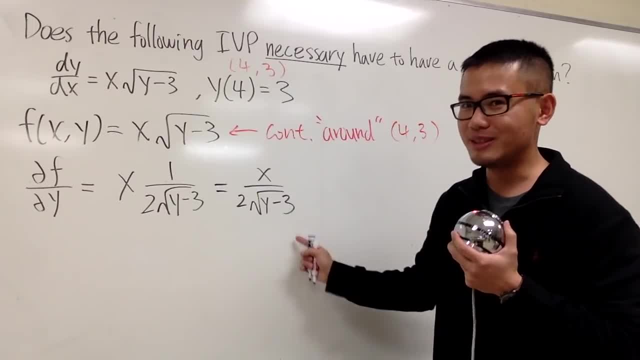 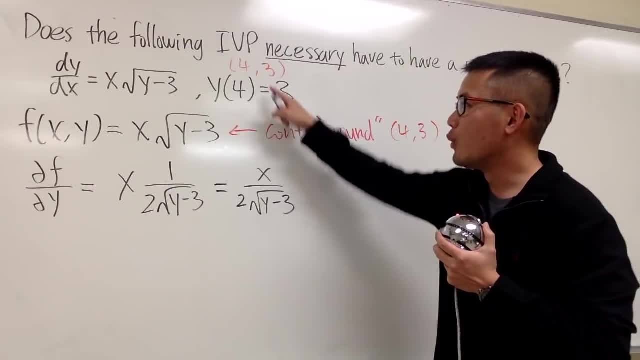 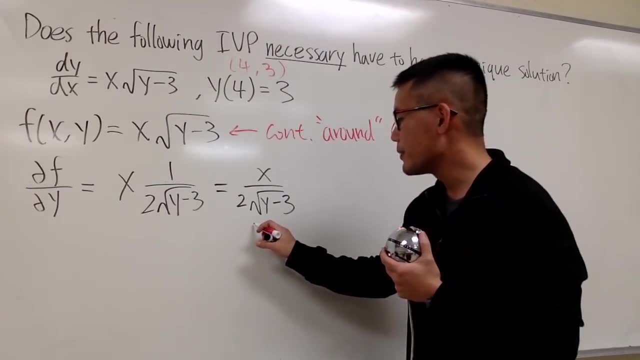 I cannot have 0 in the denominator. Unfortunately, when I plug in this point in here, it's not defined. Therefore this is not continuous. And let me write down what I said earlier: When I plug in 4 into x, we have 4 on the top. 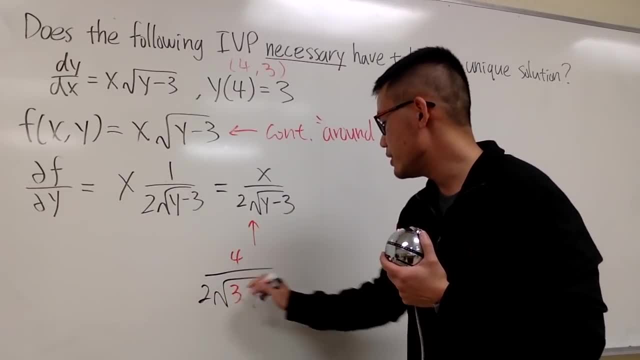 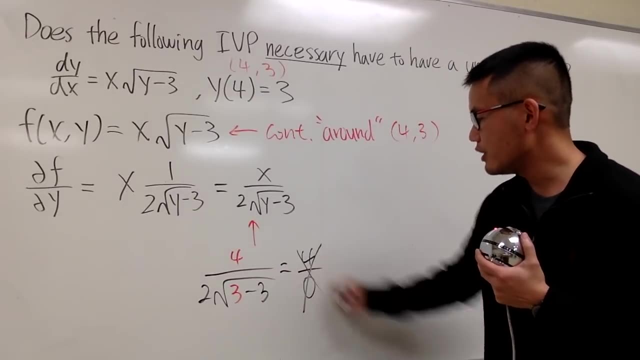 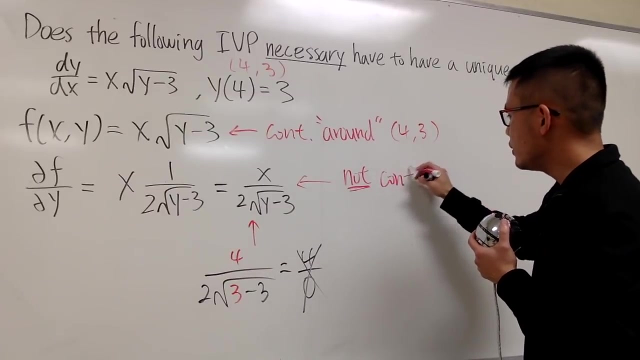 over 2. square root of y is 3 minus the 3, right. All in all you get 4 over 0, which is not defined right. This is no good. That means this right here is not continuous around 4, 3.. 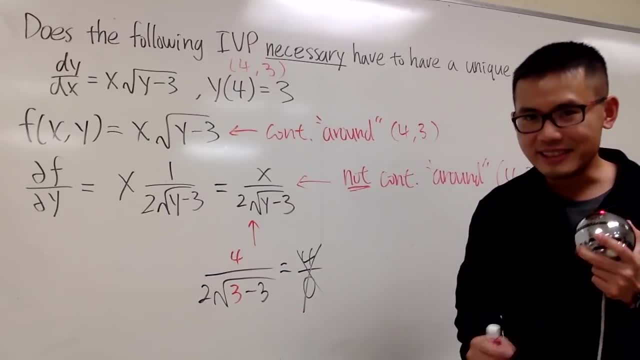 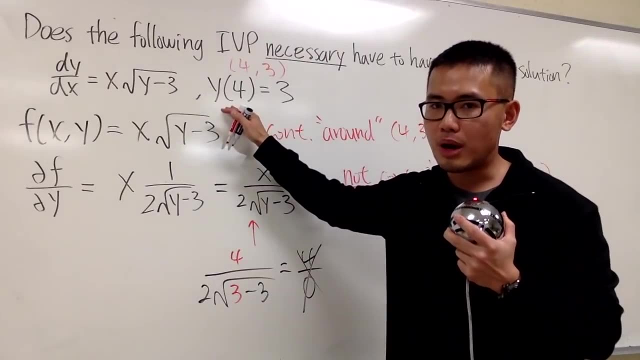 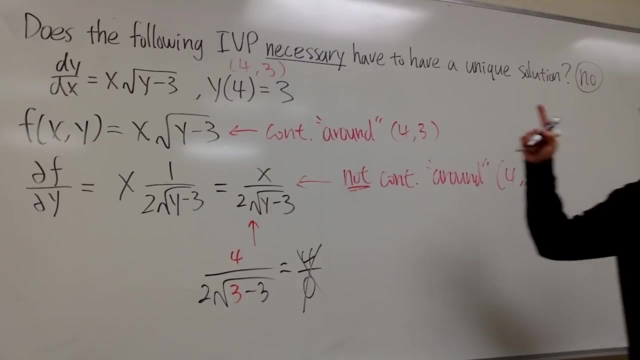 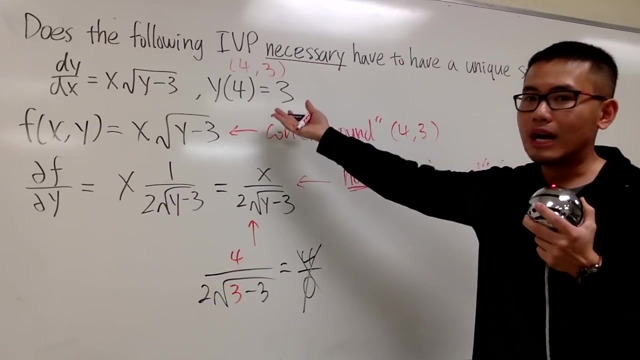 So, unfortunately, the existence and uniqueness theorem fails. We cannot guarantee that this initial value problem has a unique solution. So the answer to this is no. The answer to this is no, And let me ask you guys this: Does it mean that we don't have a solution to this? 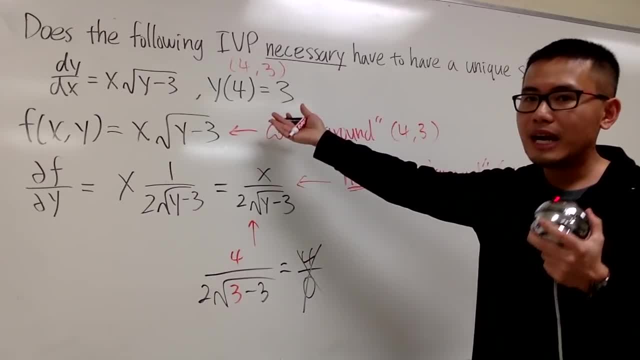 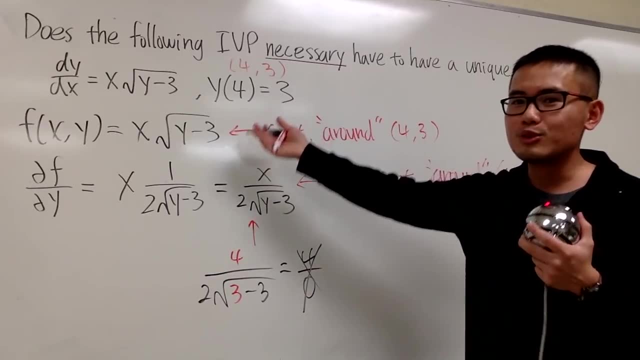 No, it doesn't okay. Does it mean that we necessarily have to have 2 solutions to this? No, cannot guarantee that either. Does that mean that we have 3 solutions or 4 solutions, or whatever? I cannot guarantee that either. 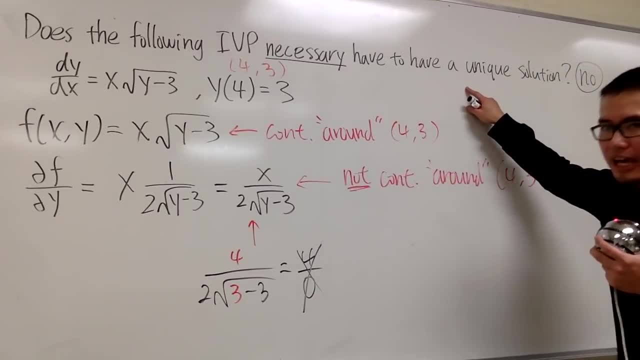 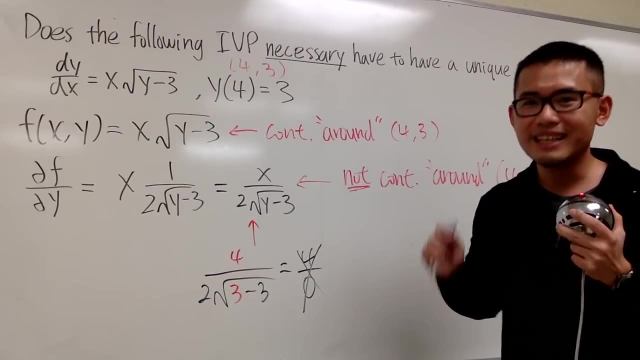 All I can guarantee is that I cannot say this right here has a unique solution, But could I still have just one unique solution to this? Yes, it is possible, okay, Yes, it might still be possible, but I just cannot tell you at the moment. 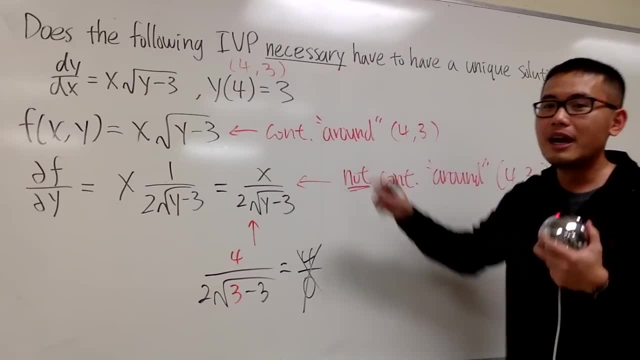 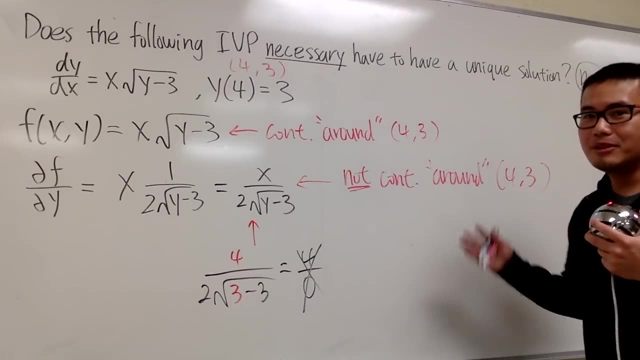 So I cannot promise. That's why I put down unnecessary. I just cannot promise you that this equation has a unique solution at the moment. okay, And let me just convince you guys real quick that how many solutions we have. Let me just show you guys real quick. 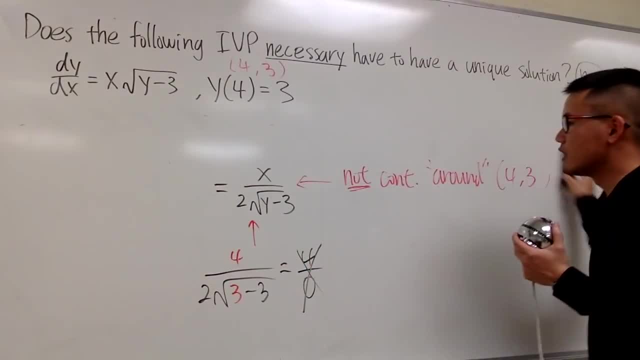 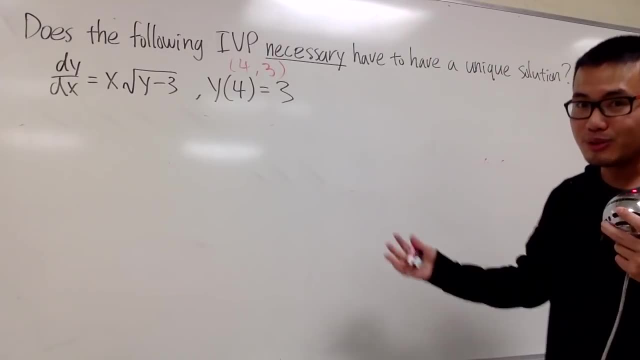 So now I will just kind of go through this. I will solve this. I may still just end up with one solution, I don't know. I may end up with no solution. I may end up with 3 solutions, Who knows? 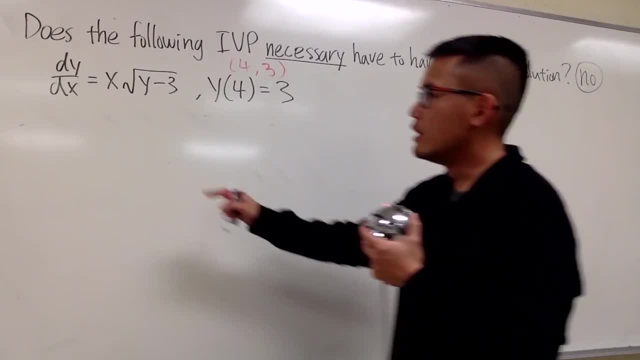 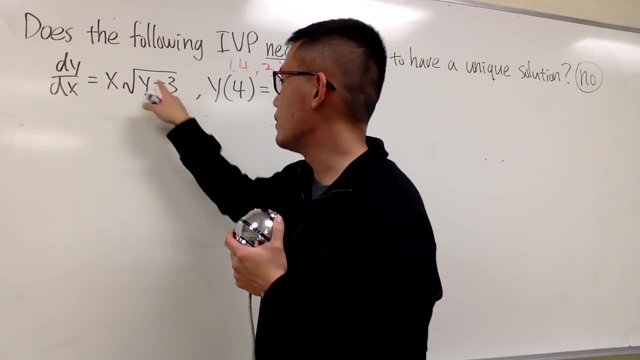 And anyways, let's just get to work on this. okay, So to solve this we can just separate the variables. I will just multiply dx on both sides and divide the square root of y minus 3 on both sides, right? So it will look like 1 over this. 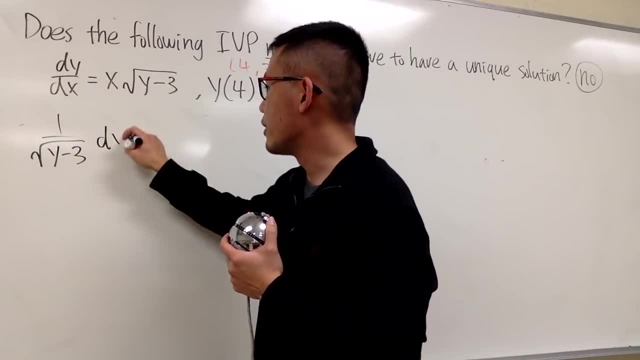 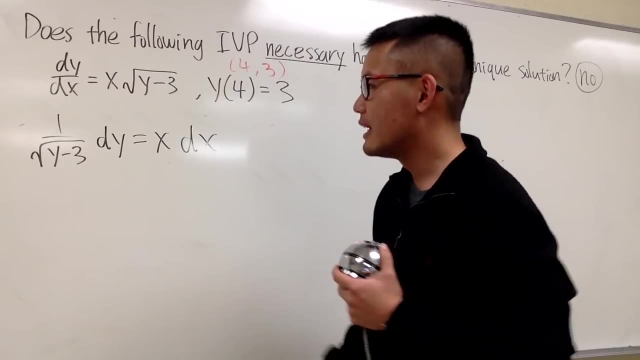 Which is square root of y minus 3.. And we have the dy right here, And this is equal to x, still here, And we multiply the dx right here. So that's what we have, okay, And now we can just integrate both sides. 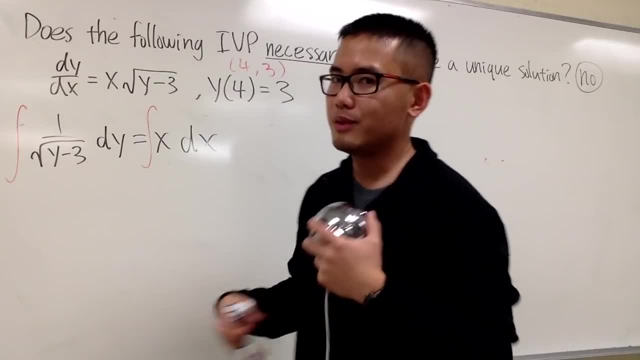 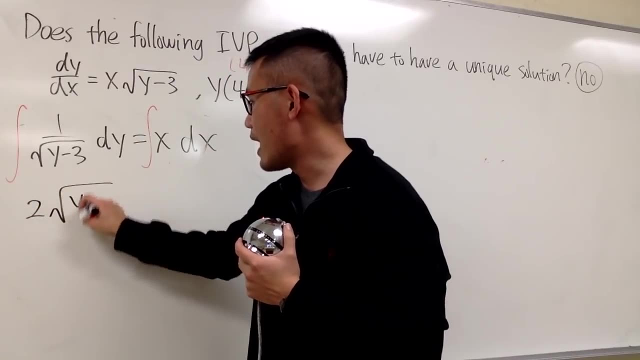 Integral of 1 over square root of y minus 3.. You can just do some new substitution, Whatever you want. Just integrate this. You will end up with 2 square root of y minus 3. And you don't need to worry about the plus c. 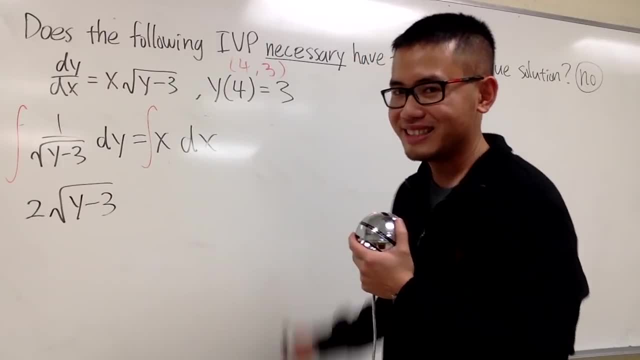 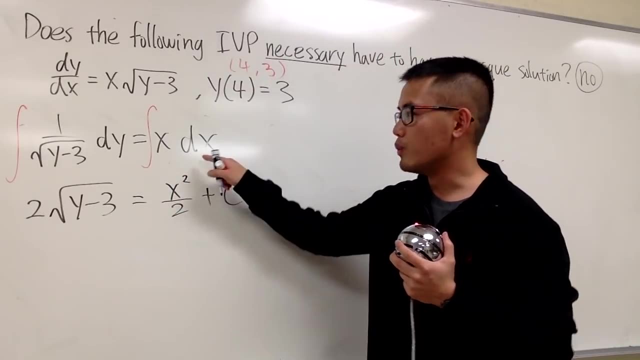 Okay, Just worry about that on the right-hand side And integrate this. You get x squared over 2 and then plus c. So this is what we have. We integrated both sides already, And let me plug in the initial values right here. 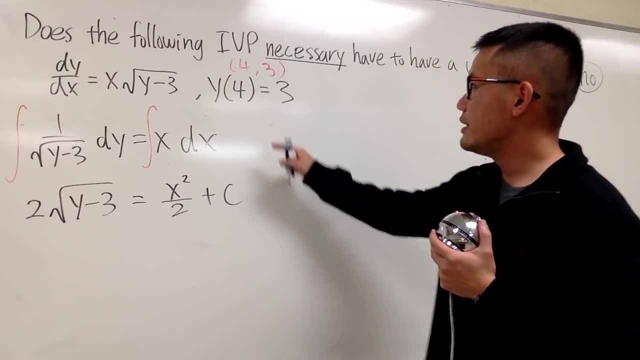 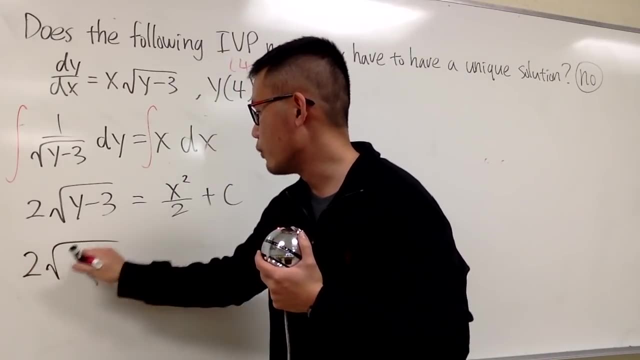 So I can solve for c right away And let me just put down 4 for x and then 3 for y. So this is going to be 2 times: the square root of y is 3 minus this 3.. And then we have this. 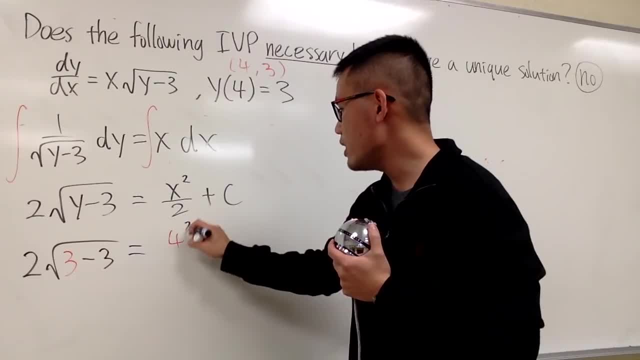 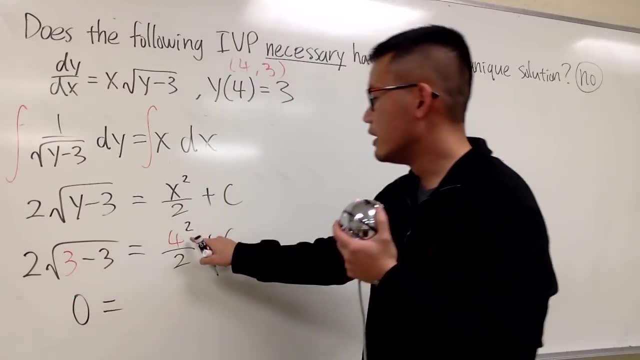 This is equal to 4 for x. So we have 4 squared over 2 plus c. On the left-hand side. all in all, you will get 0.. On the right-hand side, 4 squared is 16.. Divided by 2 is 8.. 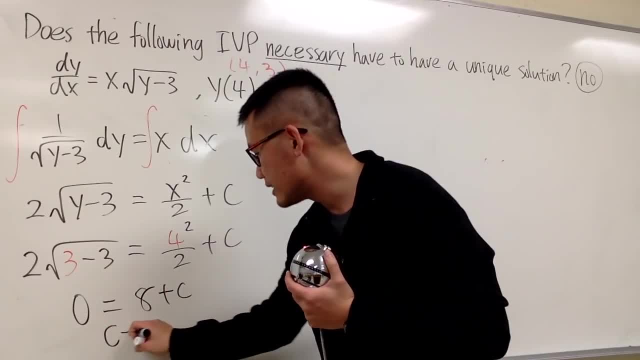 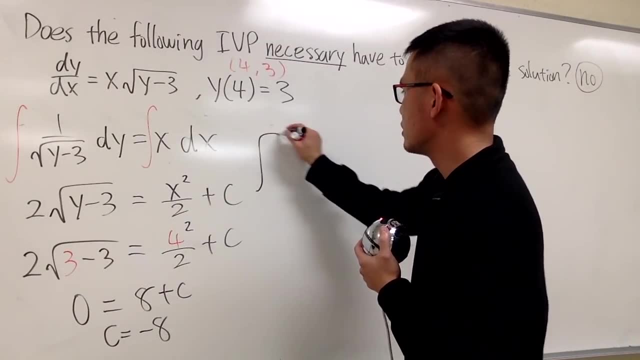 And then plus c, So altogether you see that c has to be negative 8.. Okay, And we have a solution, And I'll just write this down right here. We have 2: square root of y minus 3 is equal to x squared over 2.. 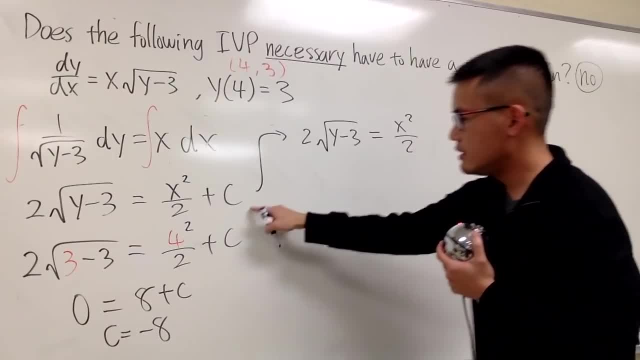 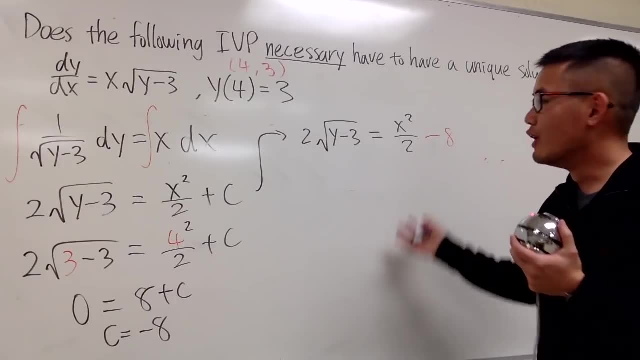 Okay, Over 2.. And the c that we found out, which is negative 8. That's what we have, And usually, whenever possible, we want to isolate the y, So we'll do that real quick right here. Okay. 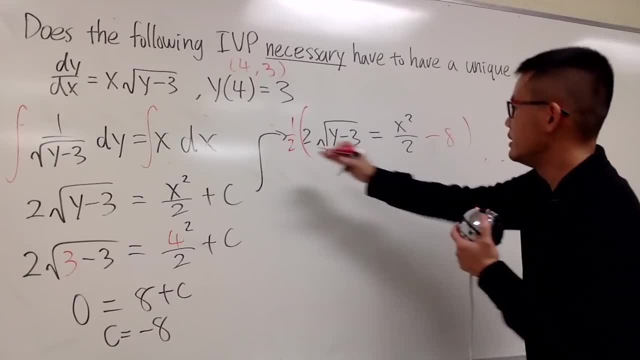 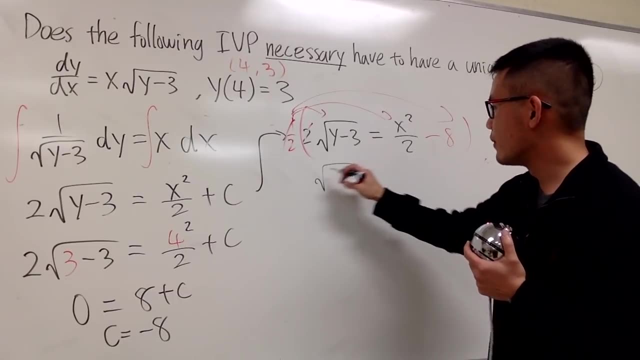 So let's multiply everything by 1 half throughout this equation. So that way this and that will cancel, And then we'll just go ahead and do that, Right? So here we have square root of y minus 3. But technically I shouldn't cross this out. 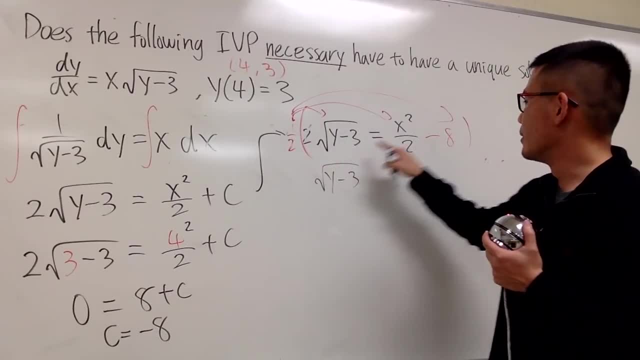 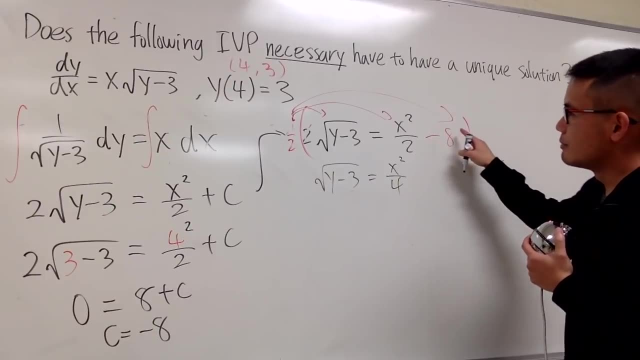 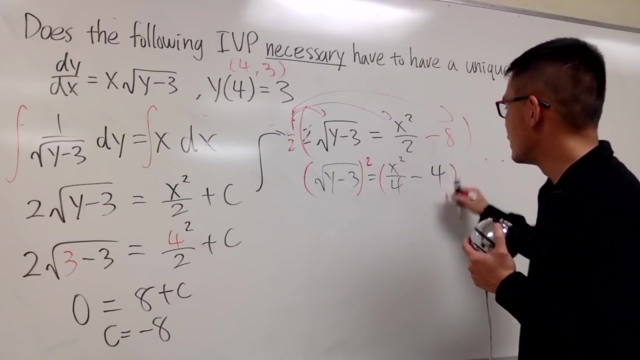 Because I still have to use the 1 half. Multiply with this, So I will get x squared over 4.. And then I will multiply the 1 half with a negative 8. So I get negative 4.. Right, And then I will square both sides. 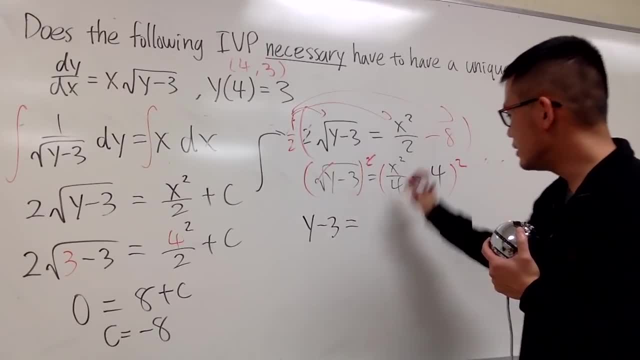 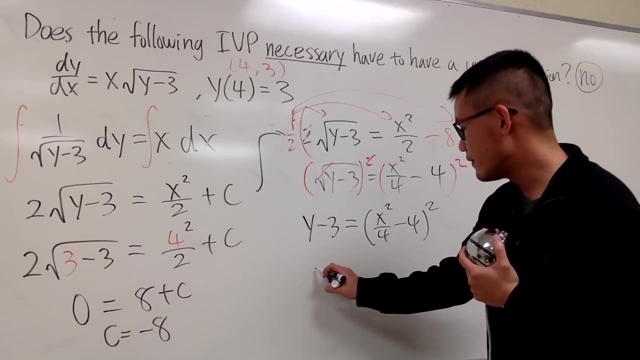 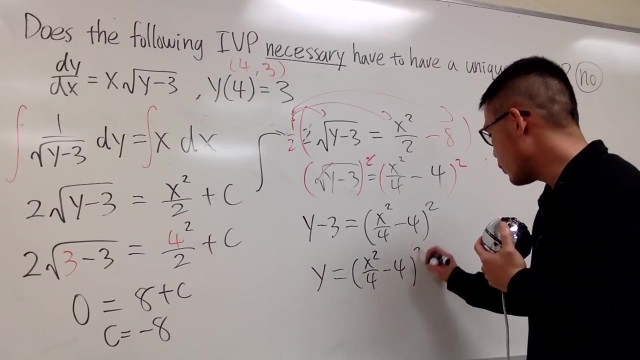 Cancel this out. We will have y minus 3 equals to this x squared over 4 minus 4.. And then square. Finally, I add 3 on both sides, So I will have y. y is equal to this x squared over 4 minus 4 squared plus 3.. 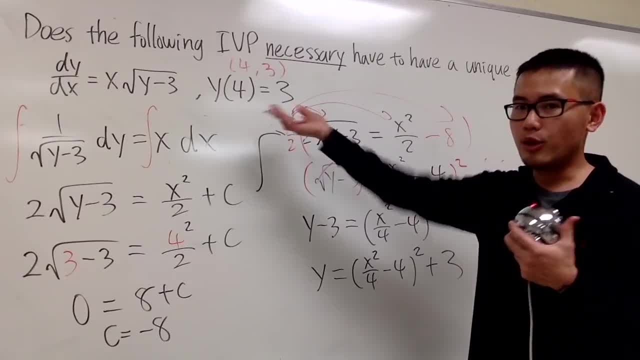 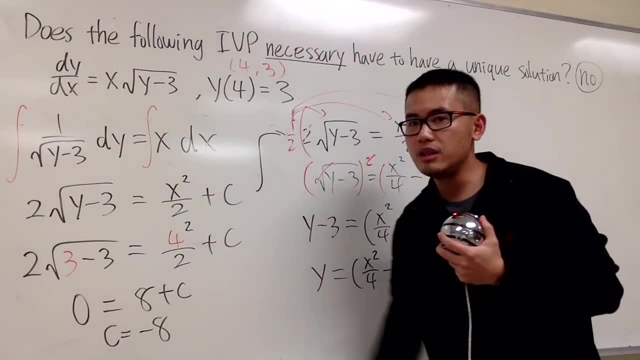 And you see, this is the solution to that. No problem, Right? So we solved the differential equation by separating the variable And we solved for the c already. So this is, of course, an answer to that. No problem at all. 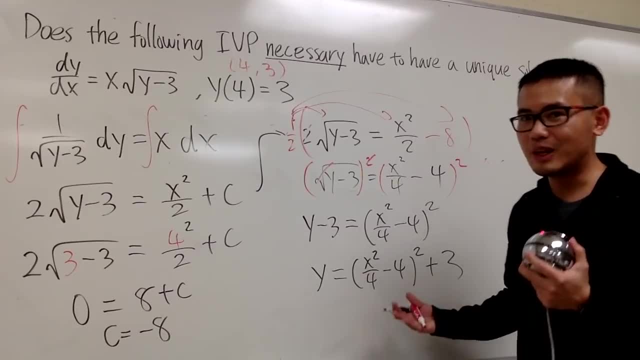 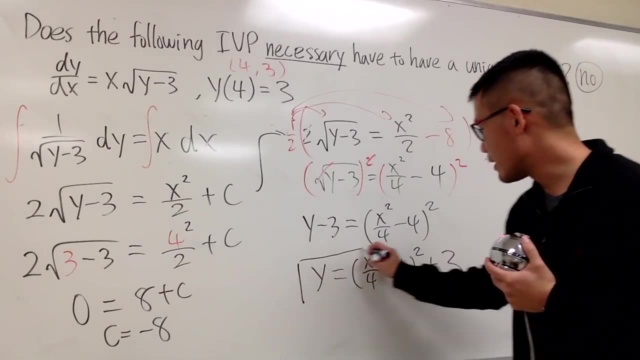 However, I will just tell you guys, this is more of the good answer that we want to find, Because this is the interesting one. It is actually a function, It changes and things like that. So right here I will box this, just to show you: this is the one that we like. 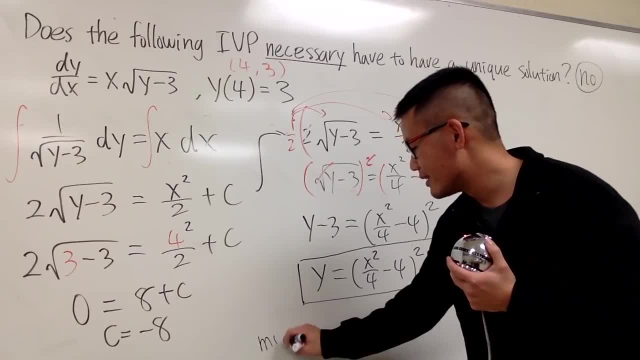 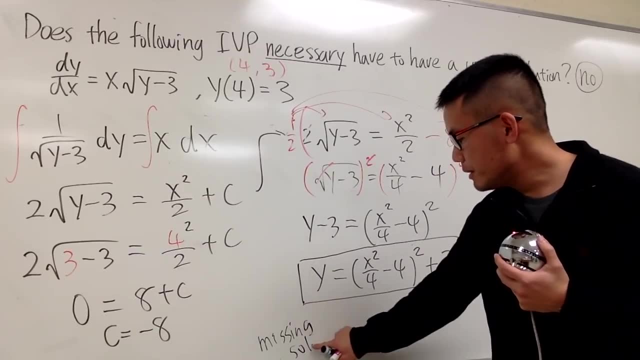 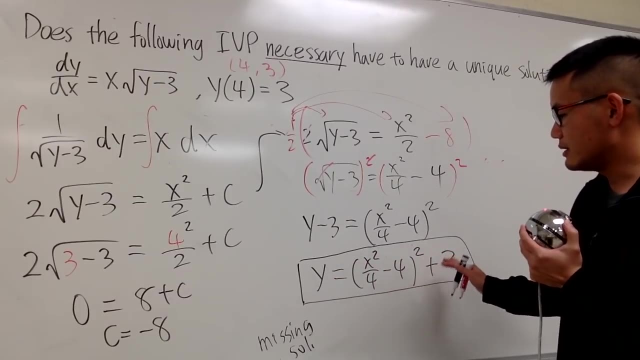 However, we do have a missing solution. OK, Missing solution right here, And what I mean by a missing solution is that it's not belong to this kind of equation. OK, It's actually a constant solution Because this, as you can see, is a polynomial equation. 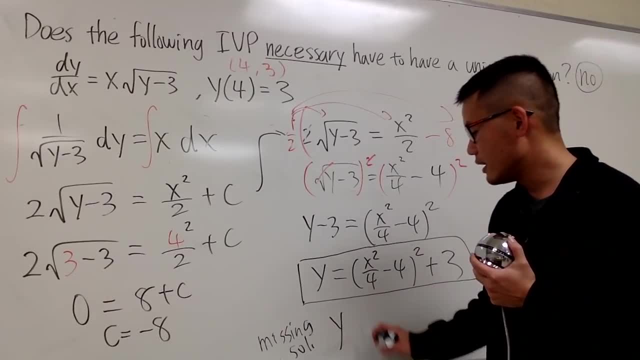 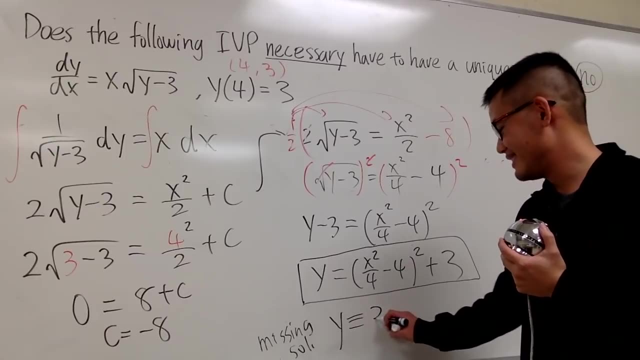 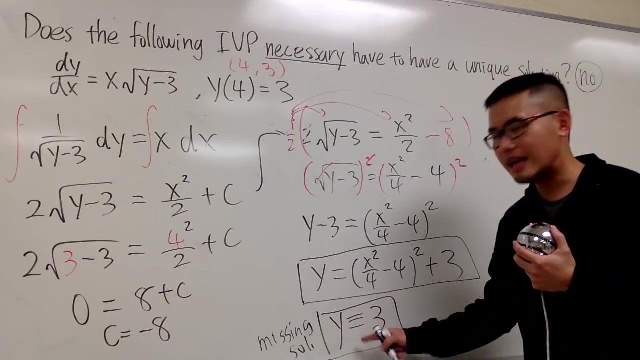 But we also have a missing solution. This is y as a function of x. OK, So I will put down identically: equal to constant 3.. This will always work. OK, This is also a solution to it. And the reason I write three lines is because I mean to say y is a function of x. 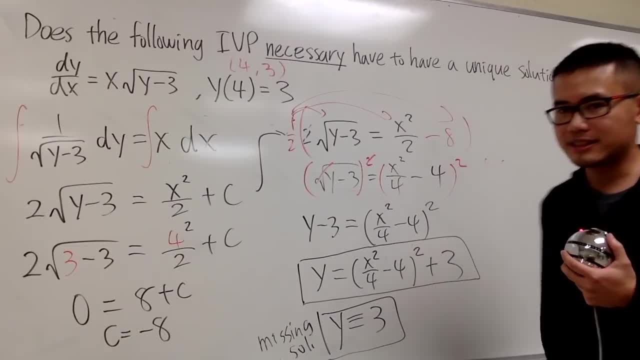 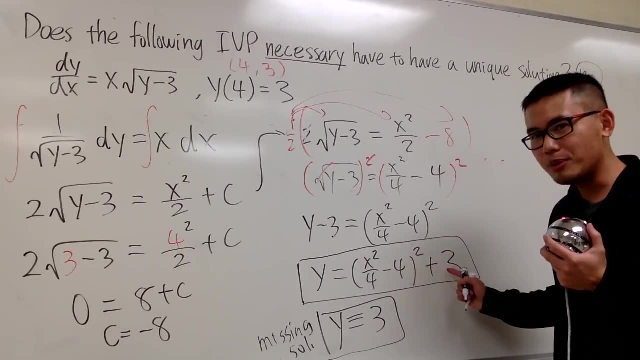 And it's always equal to 3.. For all the value of x. OK, So in fact we have one answer, two answers, And they look totally different Because this right here is a polynomial. This is just a constant. What do I mean by that? 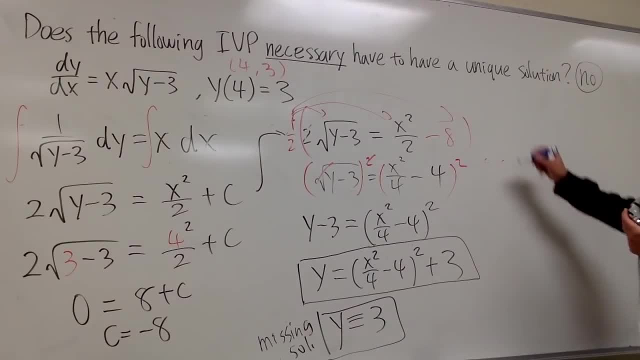 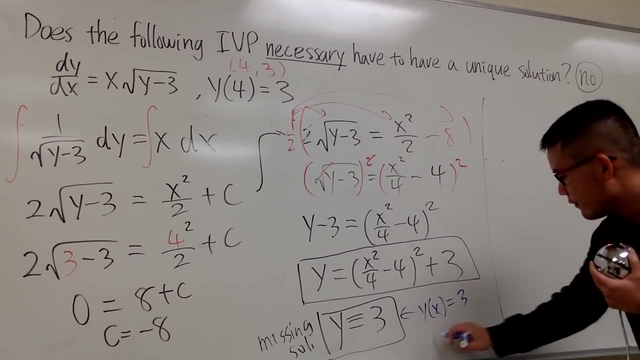 Let me just show you guys real quick. OK, Let me just show you guys real quick. So I will write this down. This is the same as saying y as a function of x is equal to 3 for all x. OK, So I will also say that y of x is equal to 3.. 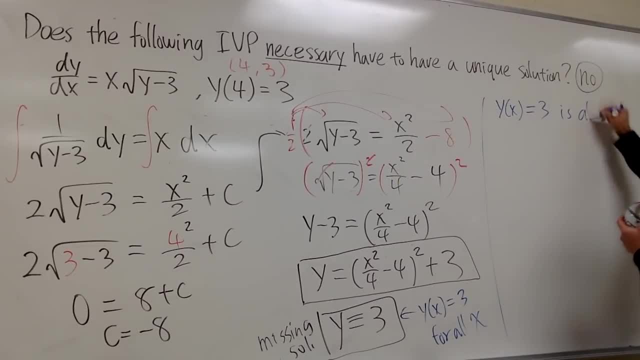 So y of x is 3 is also a solution. OK, And the reason why is because if you have this as the function, I will have to get the derivative Right. So you see that dy, dx, this is equal to 0, because I differentiate that. 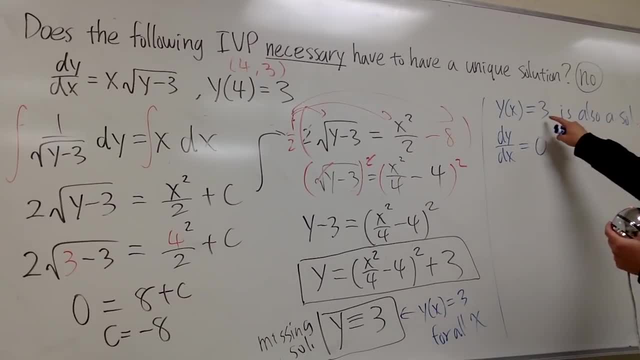 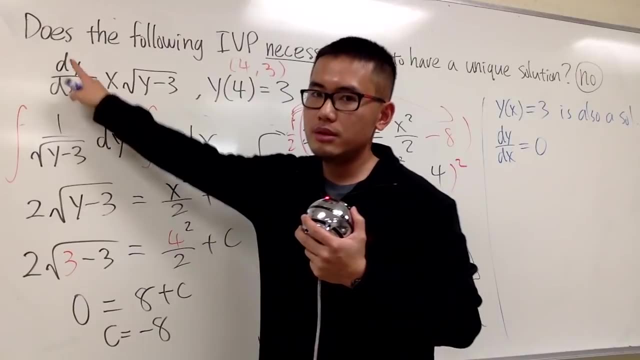 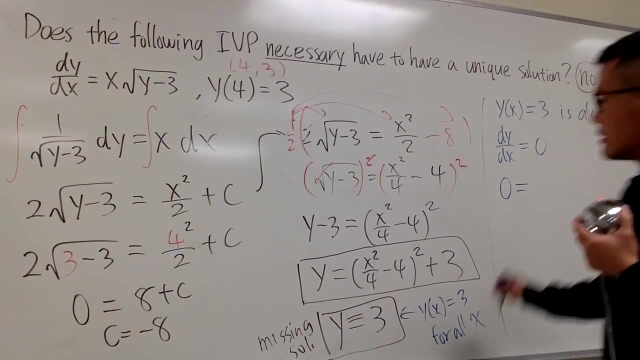 I get 0. Isn't it? And now I will plug in 3 into this y as the function And I will plug in 0 into the derivative. You will see 0 here, And this is equal to. we have the x in the front. 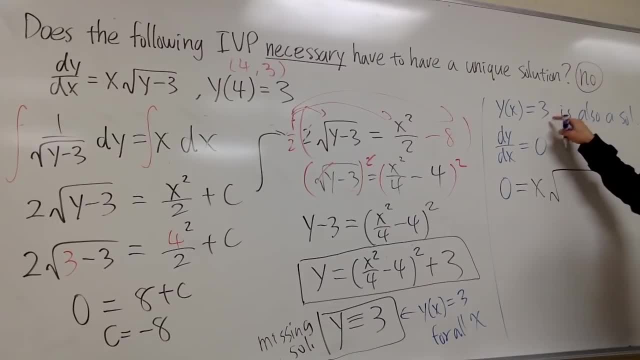 And we have the square root And we plug in the function. This is the constant function, The 3.. OK, I plug in 3 inside, Minus that 3.. And you see that this is, of course, still 0..